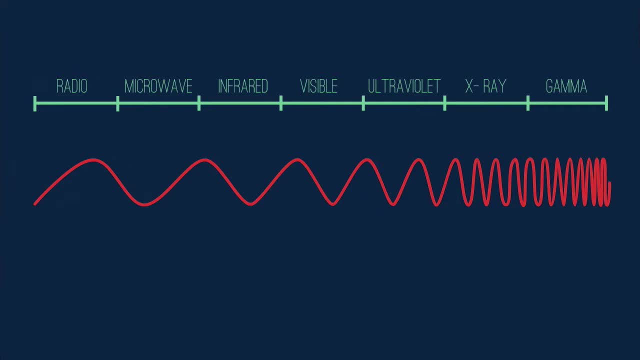 of light. Here is the full spectrum, starting with the low-energy, least harmful radio waves, then microwaves, infrared or heat radiation, then comes the rainbow spectrum of visible light, from red to violet and finally the more harmful rays, ultraviolet x-rays and gamma rays. So let's try another question: Energy from the Sun to the earth. 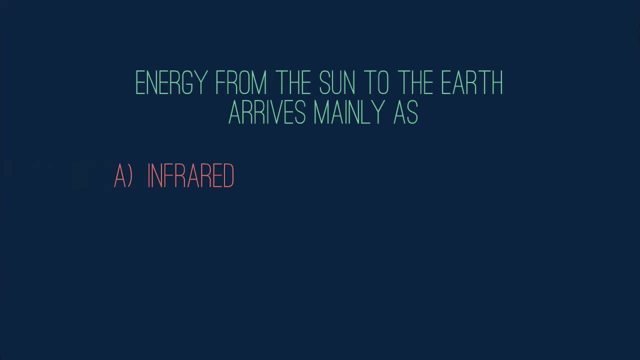 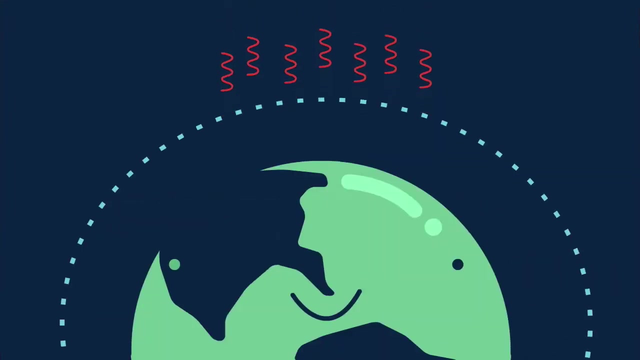 arrives mainly as infrared or heat radiation, visible light or ultraviolet radiation. Pause the video and think of your answer. Well, the answer is yes. If you pump air into a football ball and throw it into the air, you can see that there is a small amount of ultraviolet trapped in. 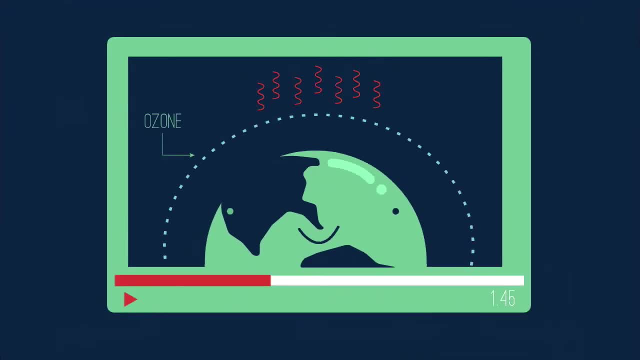 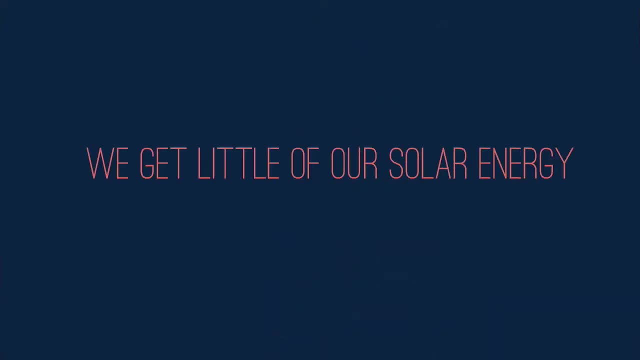 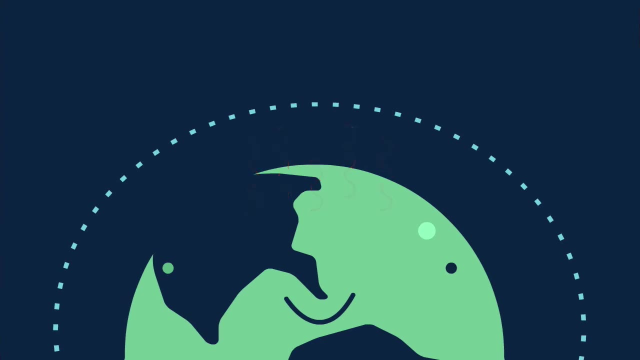 the upper atmosphere by ozone. although enough gets through to damage our skin if we stand too long in the Sun and we only get a little of our solar energy from infrared or heat radiation, The visible light gets straight through our transparent atmosphere and is partly absorbed by the earth. 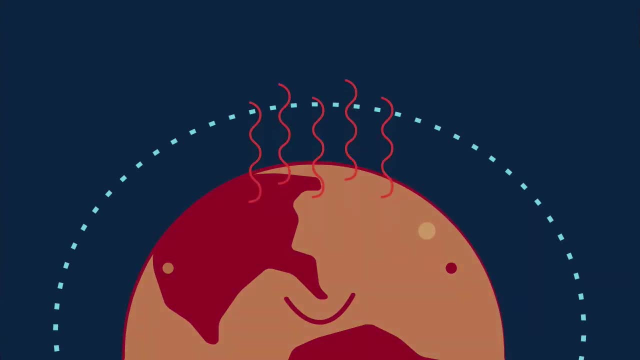 which gets hot. Now, hot is not the best way to describe the energy we get from the sun, but it is the best way to describe the heat that is produced by the sun. Now, hot things radiate infrared rays. You could try holding your hand very close, but not touching your cheek, Can you? 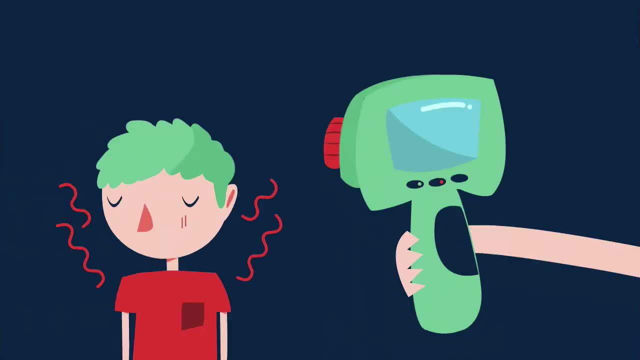 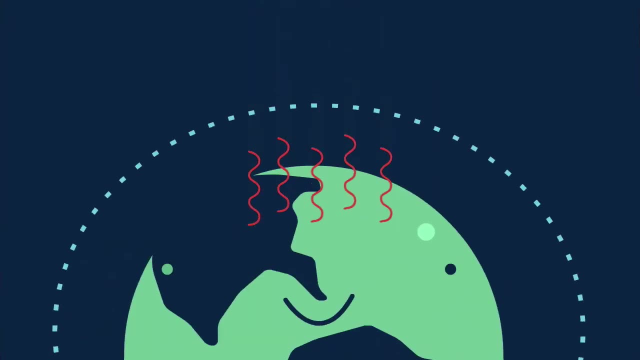 feel a glow. That's the infrared radiation. Infrared cameras can pick up this radiation emitted from warm bodies. Now here's the catch: Although visible light got through the atmosphere, the infrared radiation coming from the earth finds it more difficult to get through. 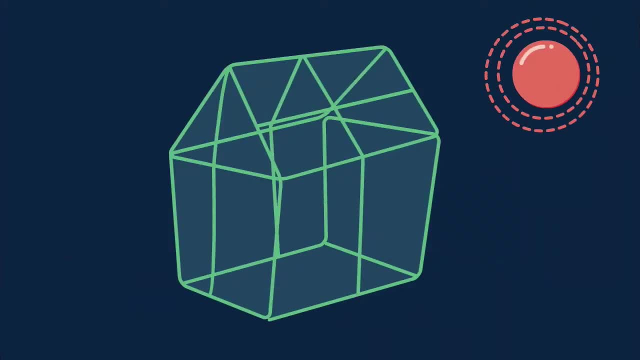 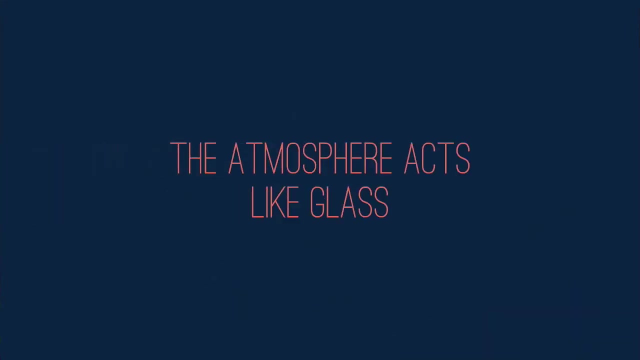 A greenhouse in the Sun, with its windows closed, works in a similar way. Visible light gets through the glass, heats the soil, which glows, giving off infrared heat. But this cannot get through the glass, so the heat builds up inside the greenhouse, So the atmosphere acts a bit like 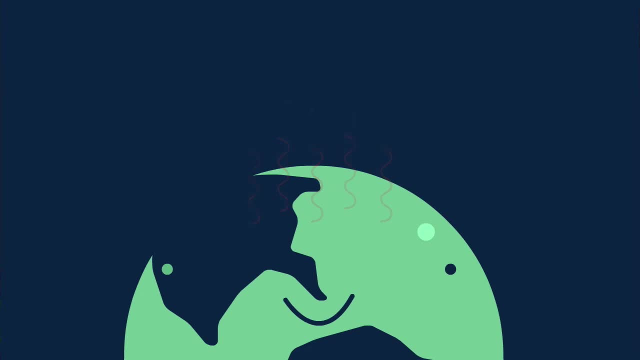 glass letting visible light through to warm the earth. But some of the heat or infrared radiation now given off gets absorbed by certain gases in the atmosphere, And these are the gases we call greenhouse gases. In this way the earth is kept warm and we say there is a natural greenhouse. 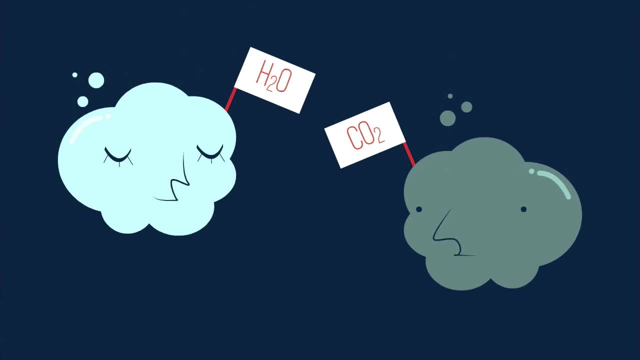 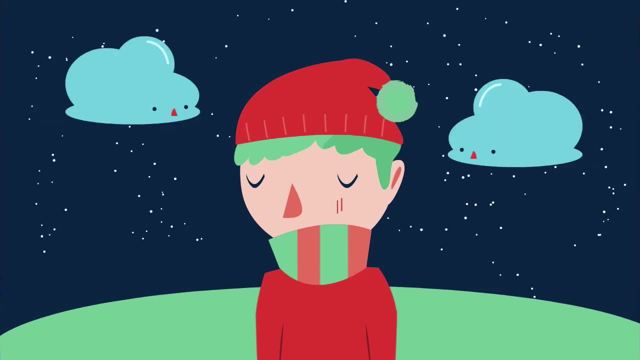 effect. The greenhouse gas is a natural greenhouse effect. The greenhouse gas is a natural greenhouse effect. The two natural gases that absorb infrared are water vapor and carbon dioxide. If you live in the colder climates, you will know that clouds made of water droplets insulate night.